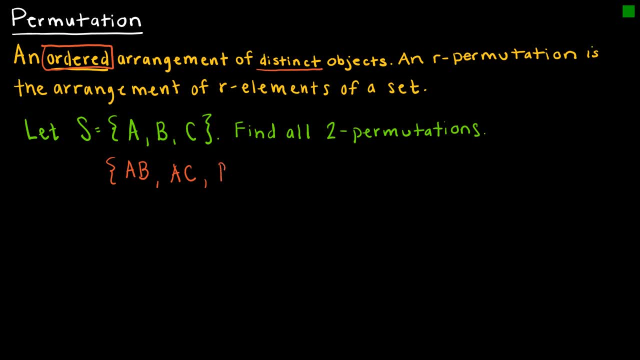 not, because again they're distinct objects, And then B A, B, C, C A and C B. So again distinct being that they're different and ordered makes a difference, because otherwise A, B and B A would really be the same thing. So obviously it's really easy for a small. 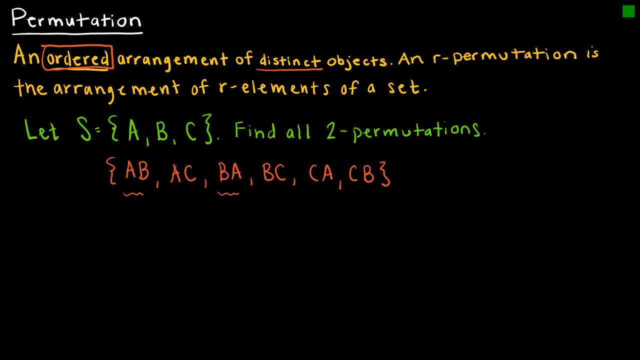 set like this, but what if I wanted to do it for a much larger set? Well then, we're going to start talking about how to use a formula, And first let's look at some of the notation: P, N, R, N. 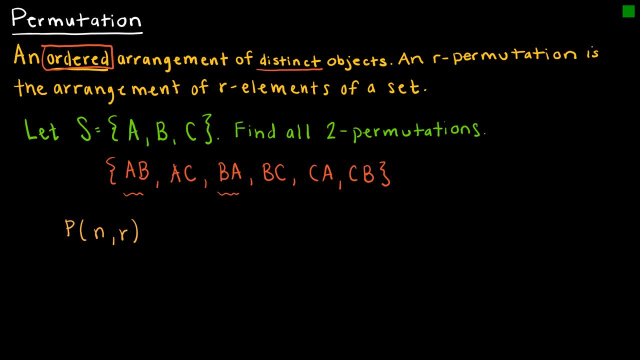 represents the number of objects in the set. So here we would have P: 3, and then R represents the number of objects that are chosen. So if it's a 2 permutation, I would choose 2.. Now I can sort. 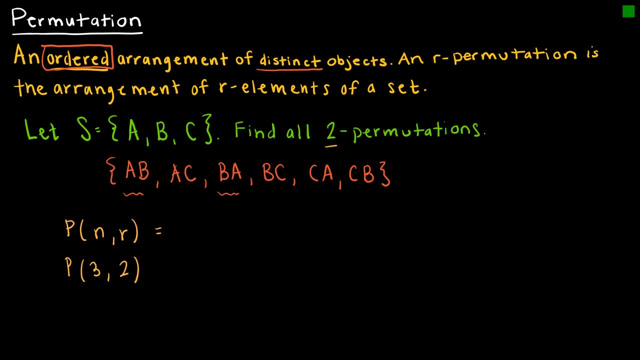 through this. but we are going to give it a formula. but I can sort of reason through it and say: well, there's three elements in the set, And so for the first position I have three choices, And then for the second position I have the two choices that remain. So 3 times 2 equals 6.. 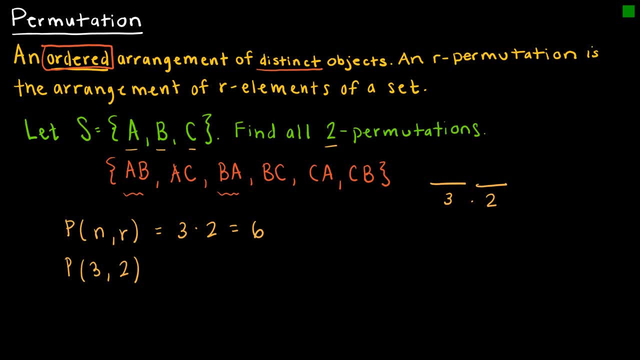 And if I didn't have to list them then I would be done. But obviously even then it's nice to have a formula that we can just plug in the values and go, And so our formula is. our formula says, because this is essentially saying that I'm going to take N times N minus 1. 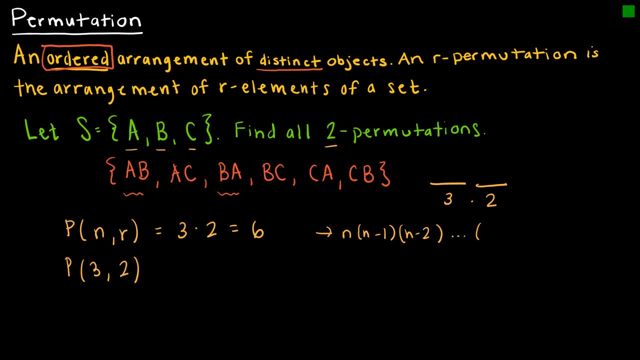 times N minus 2, blah blah blah times N minus R plus 1.. And we can turn that into a formula because basically the second is 1 less than the first, and so on and so on, and so on, until there. 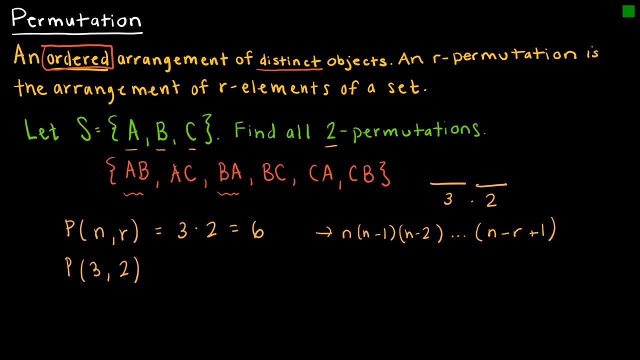 are just N minus R minus 1.. And so we can just plug in the values and go, And so we can just remember that would be N minus R minus 1, which is where we got the plus 1 because we distributed the negative. And essentially what we're saying is that we can write this: N choose R as N factorial. 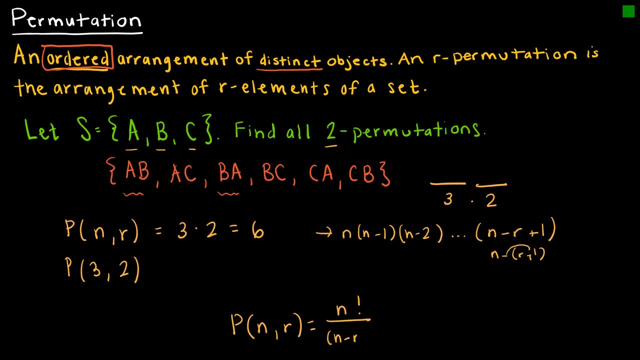 over N minus R minus 1.. And so we can write this: N choose R as N factorial over N minus R minus 1.. And so we can write this: N choose R as N factorial over N minus R factorial. So again, let's take a. 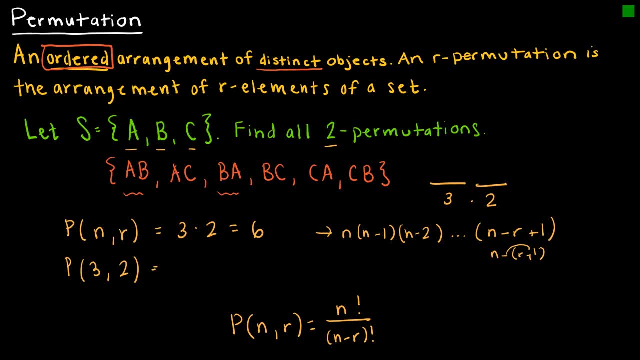 look at that using this formula. So 3, 2 would say I'm going to take 3 factorial divided by 3 minus 1, 3 minus 2 factorial, which means that I have 3 times 2 times 1 over 3 minus 2, which is 1. 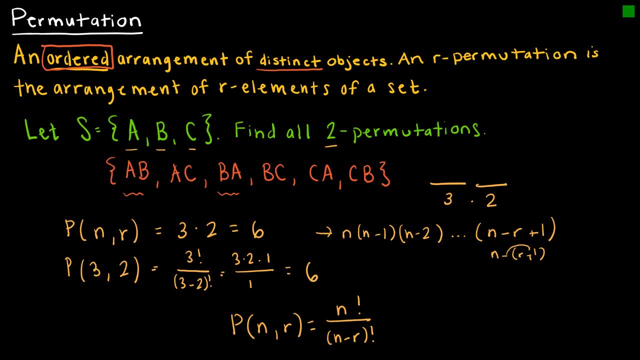 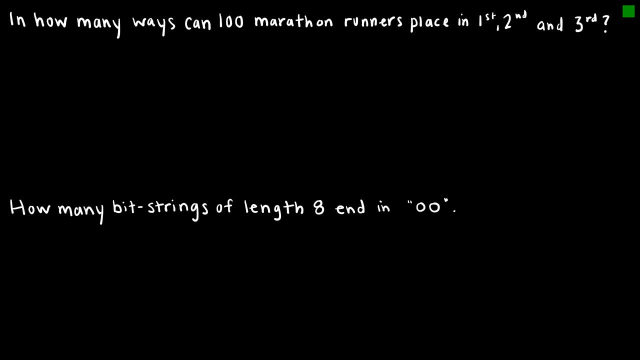 factorial, And that did give me the same answer. So let's look at a couple of practice. And how many ways can 100 marathon runners place in first, second and third? So if I weren't using the formula, I would just say, well, there's 100. 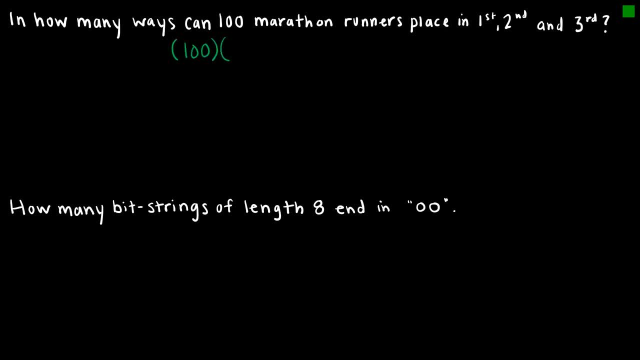 people who can be first place, And there's 99 people left who could be second place, And there are 98 people left who can be third place. And again, this one's not very difficult to figure out if I just get my calculator out, But instead let's get into the formula. So let's look at a 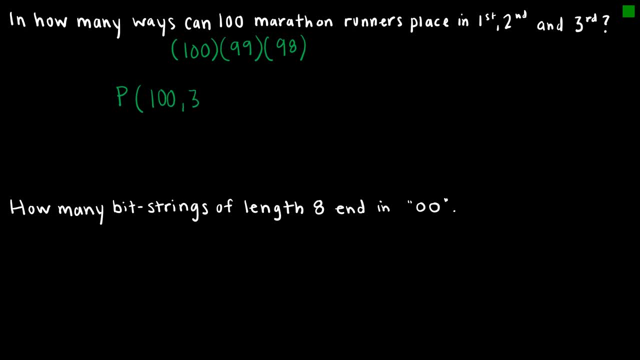 habit of saying: this is 100, choose 3.. And that tells me to take 100 factorial over. then I'm going to take 100 minus 3 factorial. Now why does that help me? Or why does that give me the? 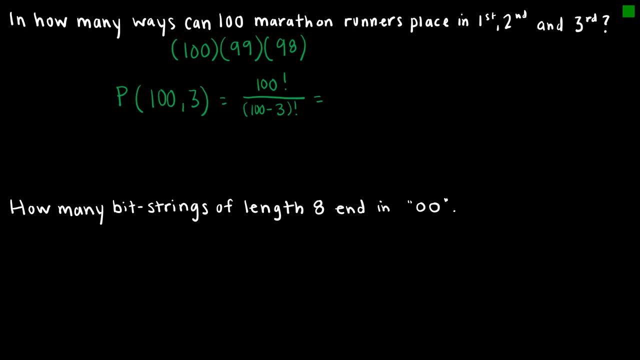 right answer, Because the numerator is 100 times 99, times 98, times 96. And I'm going to take 100 times 97, dot, dot, dot all the way down to 1.. The denominator 100 minus 3 is 97. So this is 97. 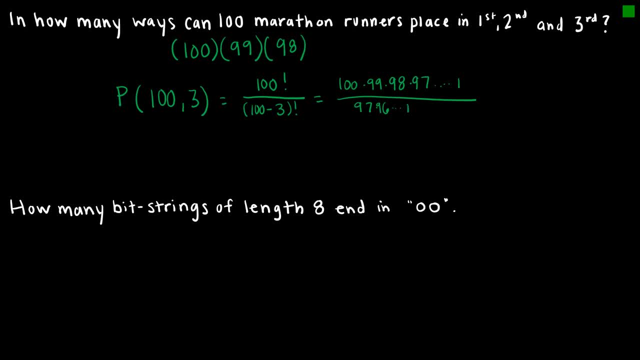 times 96, dot, dot, dot all the way down to 1.. And so what ends up happening is all of the rest of these get canceled out, And I end up right here. So again, did that save me any time? Well, not on. 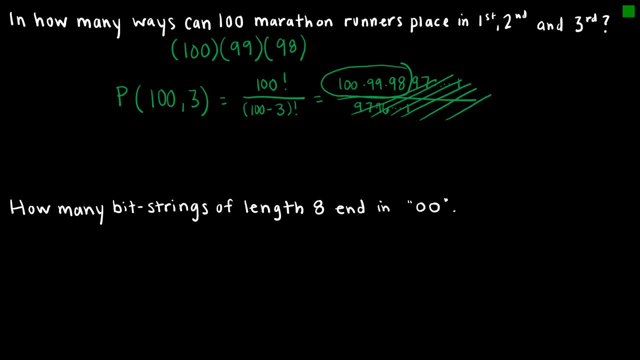 this question, not really, But on very large questions, questions with a lot of options or a lot of numbers, then it will save us some time. Plus, there's a handy dandy little button in your calculator that will do this for you. Let's look at the next one. How many bit strings of length? 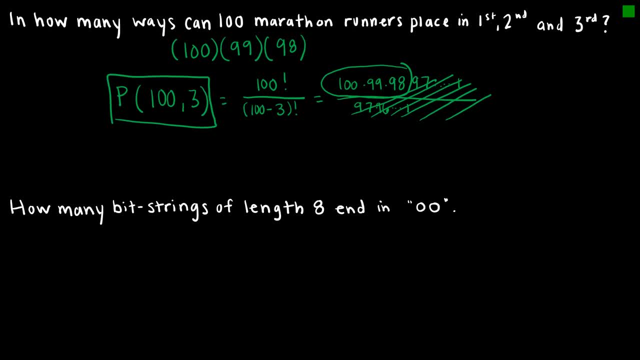 eight and in 00. So again, bit strings. this is going to be a permutation, because the order does make a difference. So again, if I have eight, eight options here and I'm saying these two end in 00, then what am I going to do here? I'm going to look at the six. 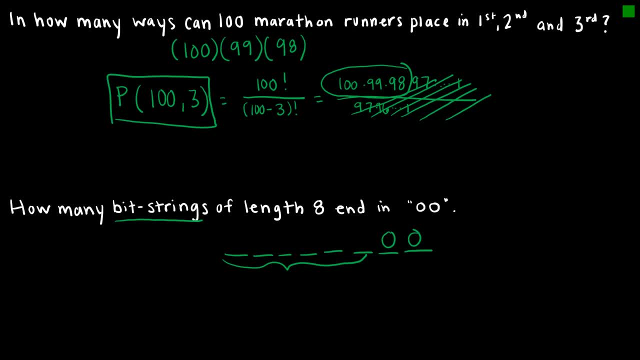 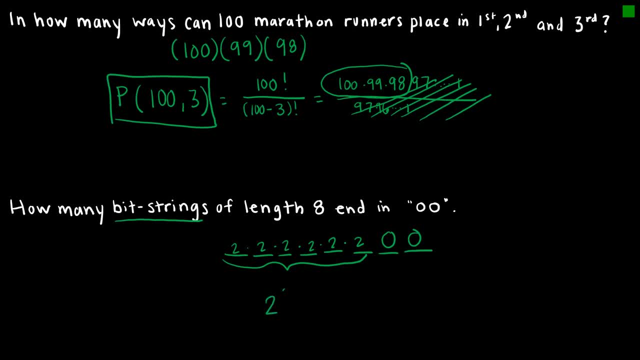 bit strings of length eight. the end in 00 is two to the sixth, because I've set this as zero and I've set this as zero And so there's really only one option for those. So it's like I'm taking. 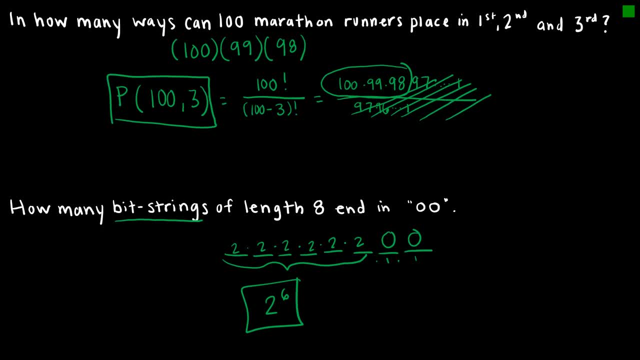 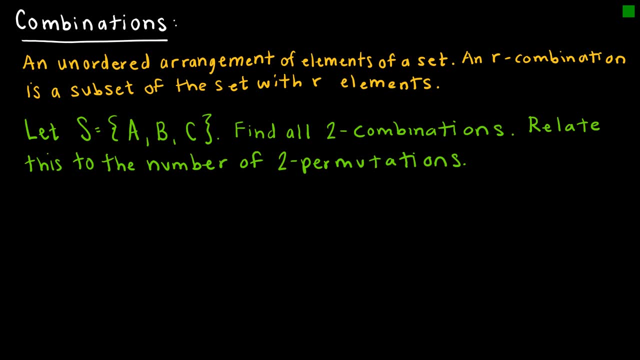 it times one, two times, So my solution would be two to the sixth. So now that we've looked at permutations, let's look at combinations. Combinations are similar to permutations, except that they are unordered, So the order does not matter. And again, 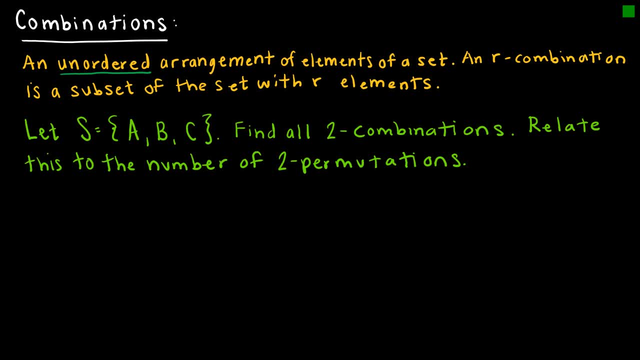 everything else is really the same. We're talking about an R combination, which is a subset with R elements. So, again, if I looked at my tiny little set ABC, if I were going to find all of the two combinations, let's start by looking at the 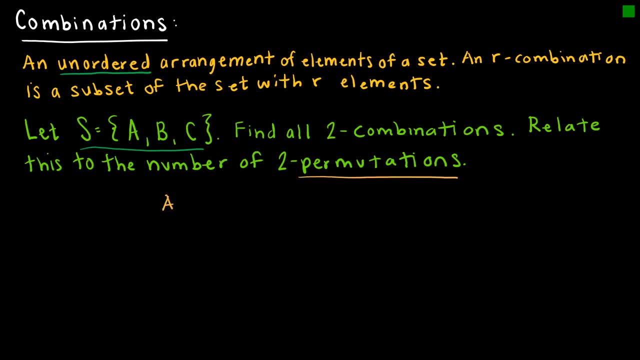 number of two permutations which we already did. So we said AB and AC, And we also said BA and BC, And that's a new one, So I'm going to write it in yellow. And then we said CA And we said CB. 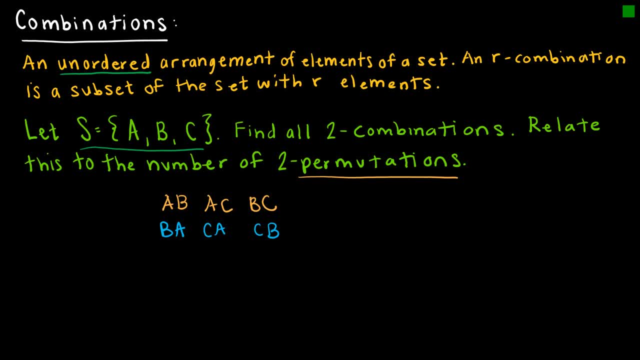 And so there are six, two permutations. But how many two combinations are there? There's only three. And why are there only three? Because we had two of everything, So we had to end up dividing by two. So our formula helps us to do just that. 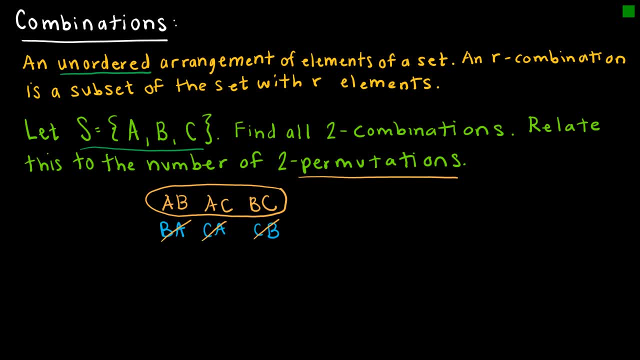 So obviously the formula is important on this one, And so my formula says I can find the number of combinations N comma R, which tells me in this case I would be finding the number of combinations of three items and I'm choosing two, And this tells me to then take N factorial. 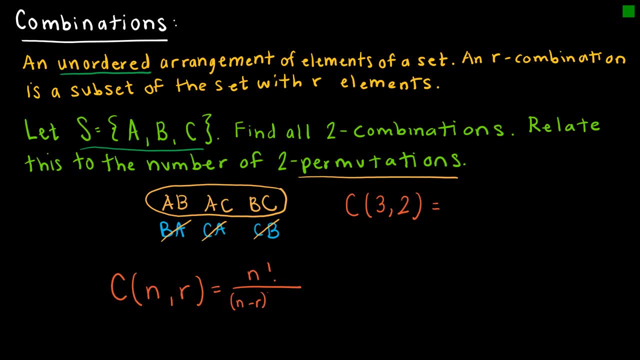 divided by N minus R factorial, just like I did before, but now I'm also taking it divided by R factorial, And that R factorial is what's going to end up getting rid of all of the duplicates. So here I'm going to take three factorial. 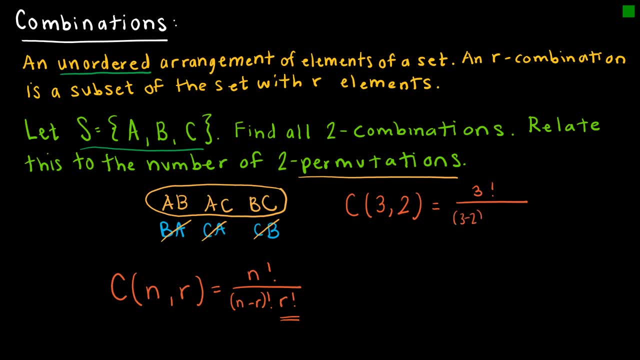 And, just like I did before, three minus two factorial, which is just one factorial but also two factorial. So this ends up being three times two times one. three minus two is one factorial, so just one, And then two factorial is. 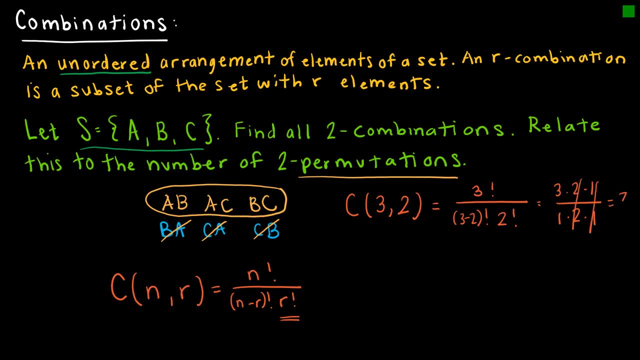 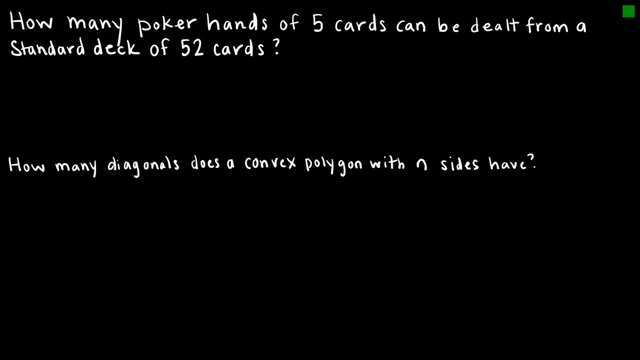 two times one And notice what happens. I end up at three because I ended up dividing by that two. essentially that got me to the answer of three, So I got rid of all of the duplicates by dividing by two. Here are a couple of practice questions for us. How many poker hands of five? 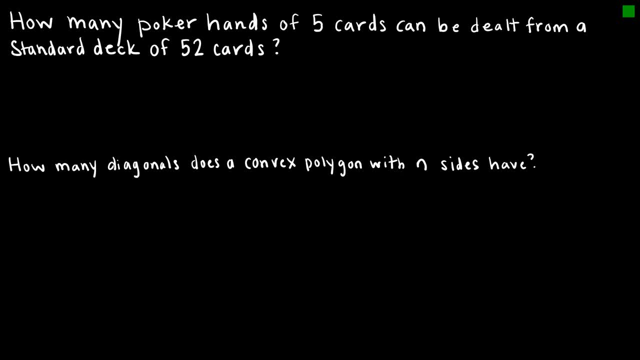 cards can be dealt from a standard deck of 52 cards. So again we ask ourselves: does the order matter? And in this case, no, it doesn't matter. So we take the number of numbers divided by two and we're going to quickly take that out and say how many people had a combination of square. 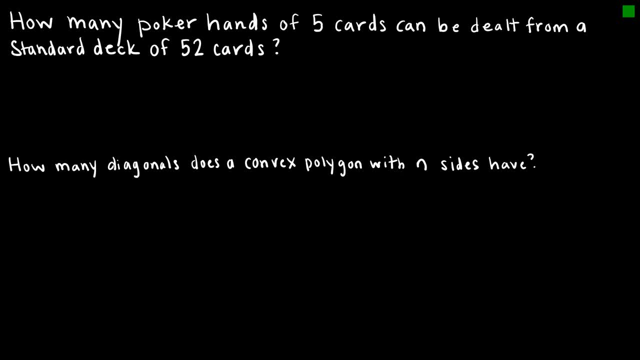 doesn't, because five cards is five cards, So it doesn't matter if I get the king first or the king last. I'm just looking at a hand of five cards. So to solve this, I would be finding a combination of 52 items and I'm choosing five of them to be in my hand, And my formula says that I'm going to 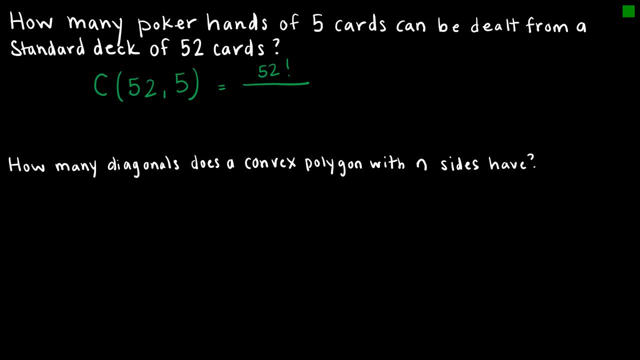 take 52 factorial divided by 52 minus 5, which is 47 factorial divided by 5 factorial. So again that ends up being 52 times 51 times 50 times 49 times 48 times 47 factorial over 47 factorial. 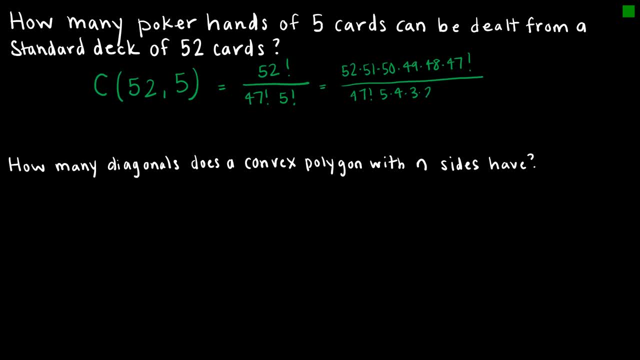 times 5 times, 4 times, 3 times 2 times, So really the whole point. there is the 47 factorial goes away, And then this denominator that's left represents the number of duplicates we would have, because we were not concerned about the order of the items, And so we end up with quite a large number, actually 2,598,960. 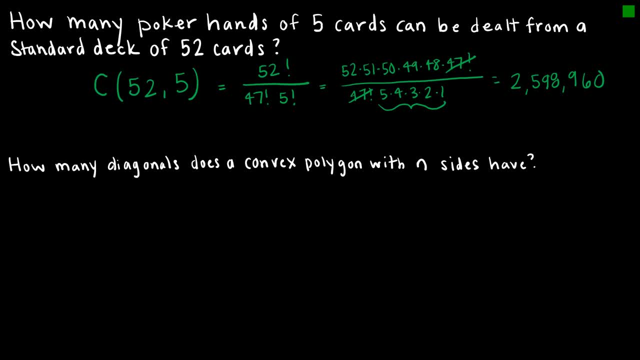 Let's look at our second question: How many diagonals does a convex polygon with n sides have? Now, keep in mind, we're not always going to be just an easy question using n or c or p. You're going to have to think about some of these. So here it says: how many diagonals does a convex? 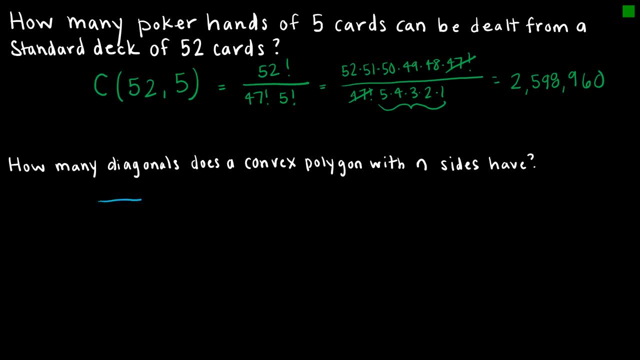 polygon with n sides have. So let's take a look at just a hexagon, So obviously a convex polygon with six sides. So let's take a look at a hexagon with six sides, So obviously a convex polygon with six sides. So if I'm looking at this vertex, how many sides, how many vertices can I connect? 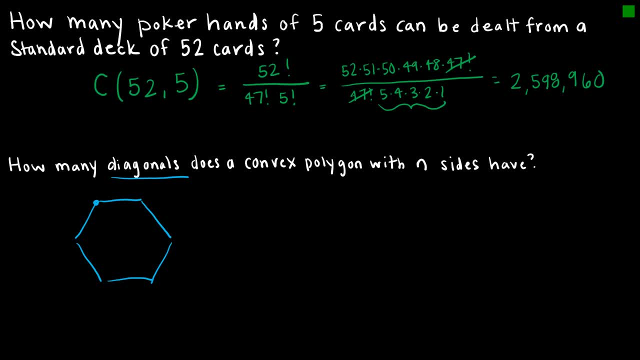 that, to How many diagonals can this one make? Well, this would take one, two, three, right? So my first has three diagonals. My second has one, two, three diagonals. Okay, My third has one, two, three diagonals. but guess what? 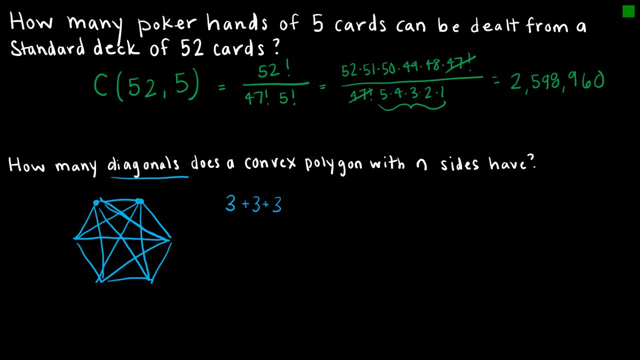